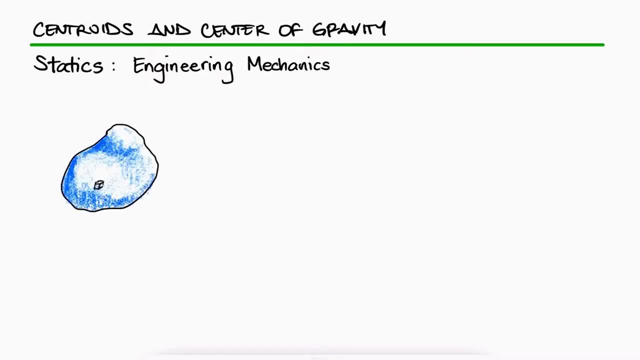 Bodies are made up by an infinite number of particles that have a weight, dw. These weights will all be oriented parallel to each other and the total weight of the body will be the sum of all the forces concentrated on a single point called the center of gravity, The location of 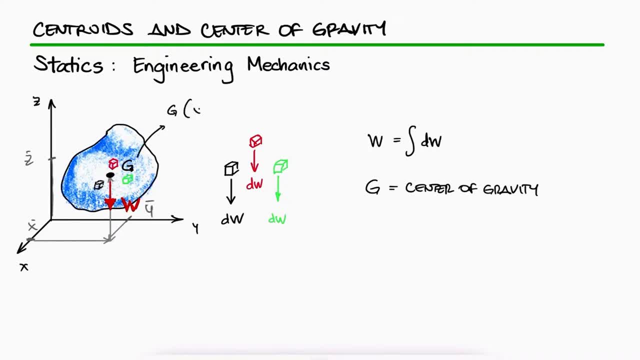 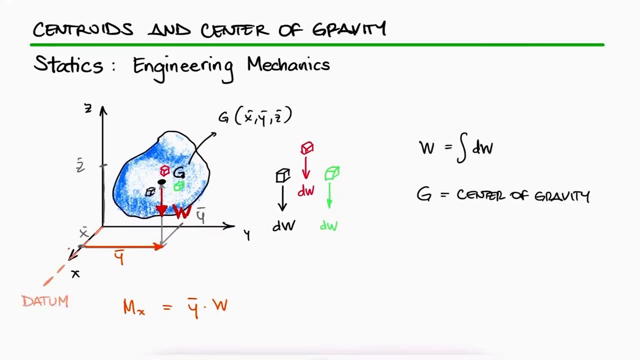 the center of gravity can be located in each of the three orthogonal directions by knowing that the moment caused by the weight from a random point of reference or datum, which would be the distance to the center of gravity, times the weight has to be equal to the sum of moments. of all the weights of the particles, which is just the integral of all the dw times the distance to each, And this is true for any direction: x, y or z. The location of the center of gravity would therefore be given in three dimensions by the coordinates x-bar, y-bar and z-bar, Just like. 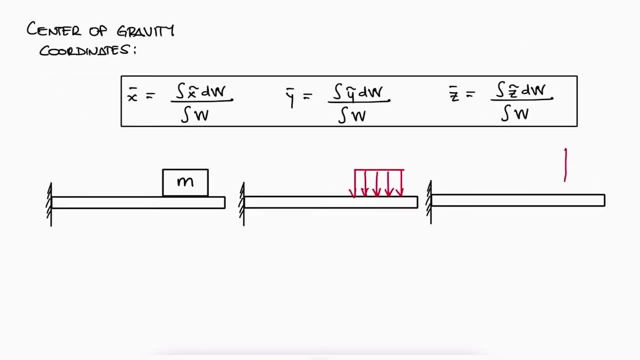 it was pointed out during the shear and moment diagrams video, a body of weight w can be substituted for a body of weight w. We can substitute it by a point load and the location of that point will be its center of gravity. For dynamics or accelerated motions of a body, we wouldn't really care about the weight. 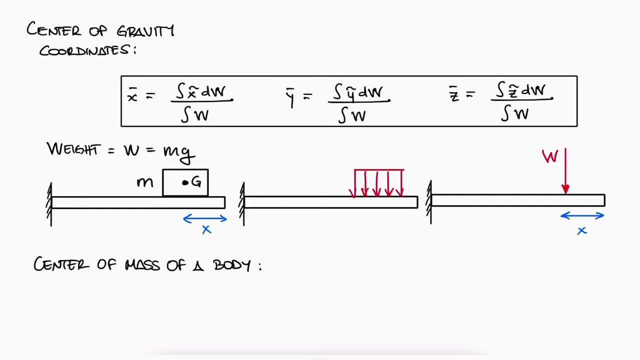 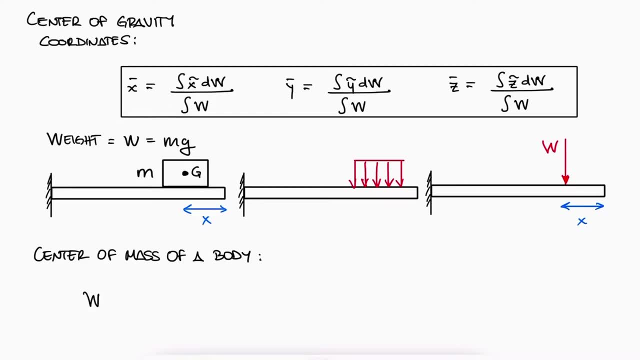 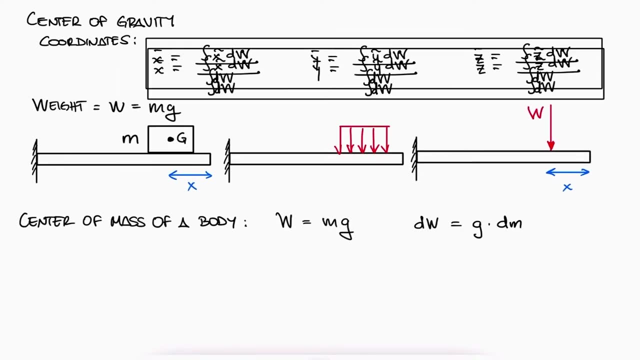 but just the mass of that particular body. Therefore, we would look at the center of mass of a body instead of the center of gravity. But since weight is just mass times the gravitational acceleration constant g, meaning that dw is equal to g times dm, we can substitute dw by gdm. 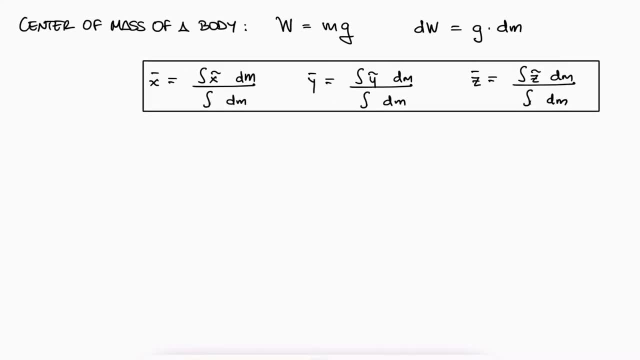 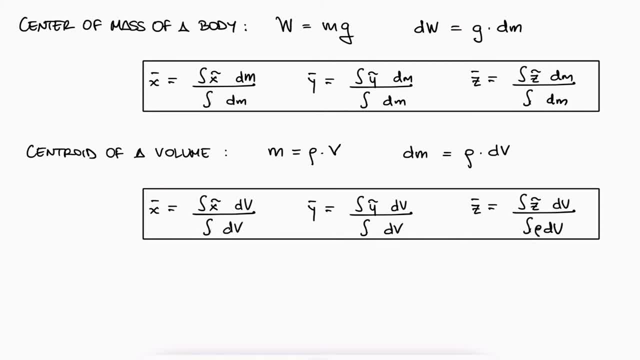 expressions substitute dm and cancel out the rows. The coordinates for a centroid of a volume would be given by the same expressions, with dv instead of dm. And finally, because a big chunk of our analyses in a static course are done with reasonable 2d representations. 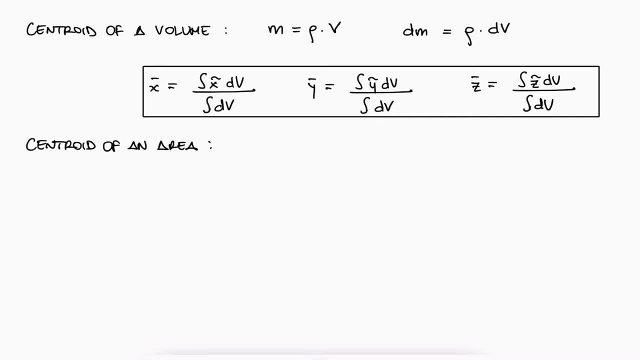 of 3d structures, it's really helpful to find the centroid of an area, assuming that the third dimension is constant throughout the load mass or volume. In this case, following the exact same procedure, the volume is z times the area, which means dv is z times da, and the expressions to: 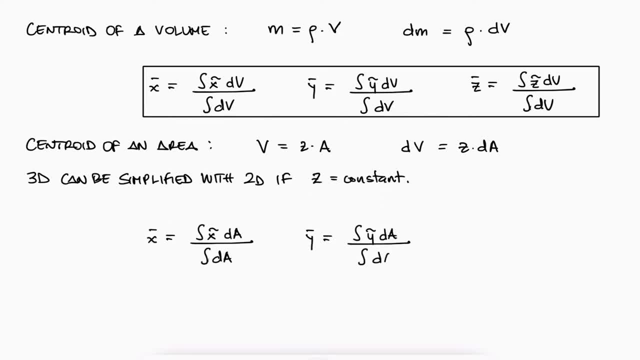 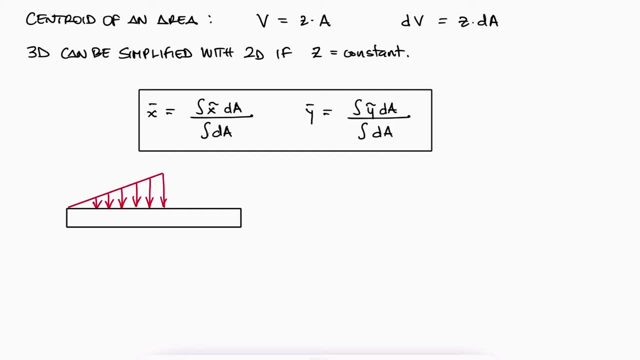 find the coordinates, have the same structure and have da instead of dv. During the last main video Shear and Bending Diagrams, I mentioned how the centroid of a triangular distributed load is used to replace that distributed load with a point load, And this was helpful to be able to. 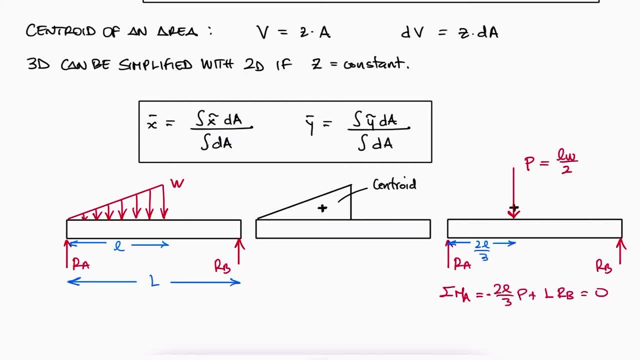 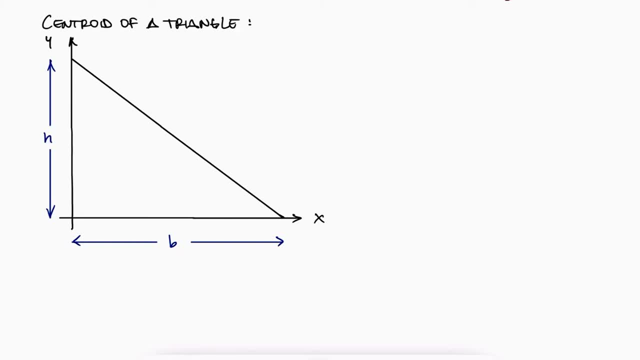 write a sum of moments and solve for a reaction force. If we want to find the centroid of a right triangle like this that has a base b and a height h, the diagonal line would be described by a straight line equation where the slope is rise over run or, in this case, minus h over b. 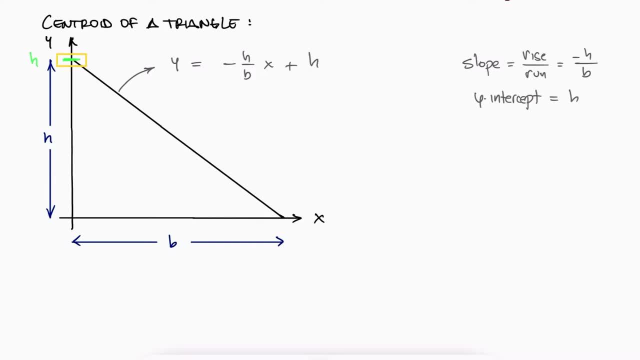 and the y-intercept is h. Solving for x, we find b over h times h minus b, which is the distance y. This tells us the width of any rectangle at a distance y. With that equation, the d-area term for that and any other rectangle can be written as x times dy, which would be b over h times h. 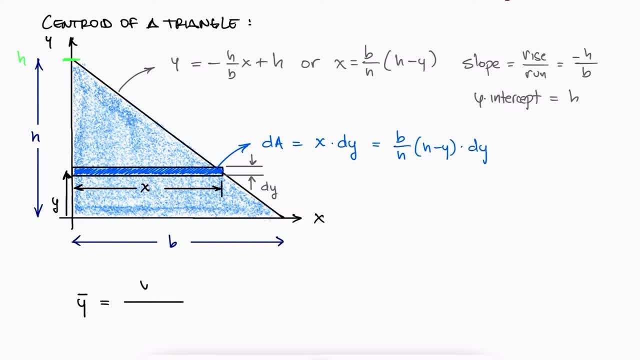 minus y times dy. Using the centroid equation in terms of the integrals and substituting da, the integral that needs to take y from 0 to h in the numerator would be 1 over 6 bh squared and in the denominator 1 half bh. This means that the centroid from the bottom, our point of 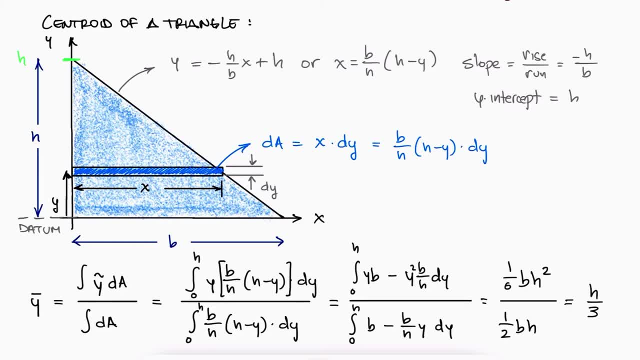 reference is h over 3.. This is what we used in the examples of the shear and bending moment diagrams, video links below. And since this process was done using variables for the base and the height, not specific unique numbers, this will always be true for any triangle. The centroid of a triangle. 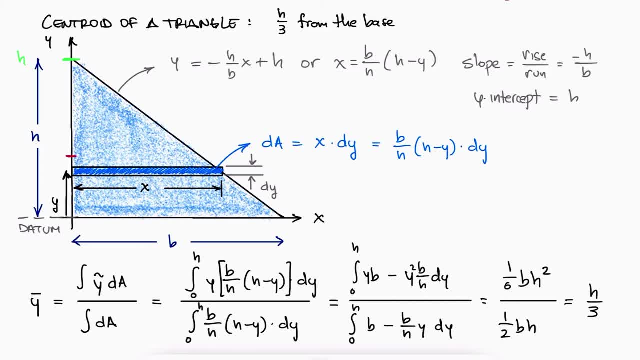 will be located at one-third the height measured from the base of the triangle, And it works for both directions. This is the same mathematical procedure we carry out for any shape that can be described by a function of x in terms of y, or vice versa If we have. 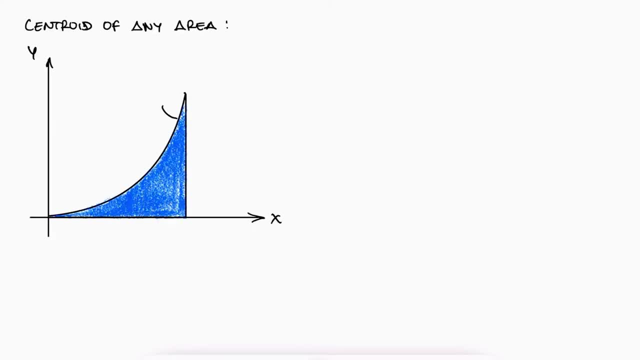 an area bound by two perpendicular lines in a parabola, from the origin to 1 comma 1, let's say meters. the da element can be drawn as a vertical or a horizontal rectangle and know that the result is going to be the same For vertical rectangles. the d-area would 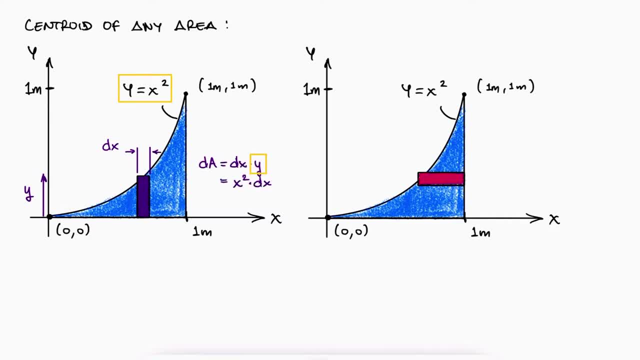 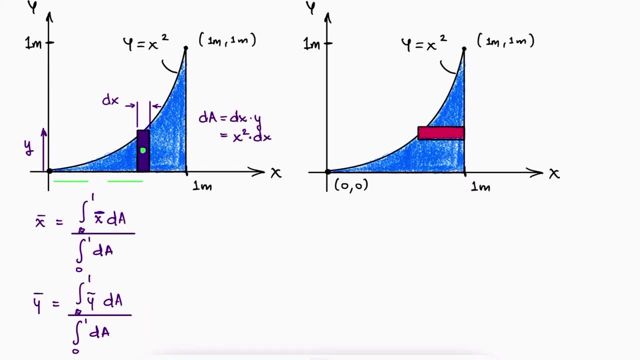 be dx times y, which is x squared times dx, and the integrals would be evaluated between 0 and 1.. The centroid of the rectangle would be at x for x bar and at y over 2 for y bar, Substituting the: 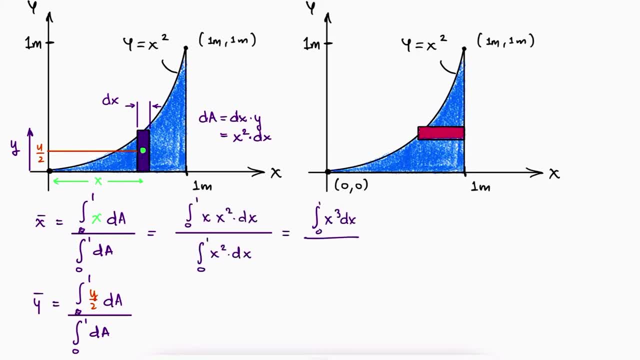 d-area, and evaluating the integrals, we find that the x-coordinate for the centroid x bar would be at 0.75 meters and that the y-coordinate for the centroid y bar would be at 0.3 meters. If we had used horizontal and horizontal rectangles, we would have found that the x-coordinate for the 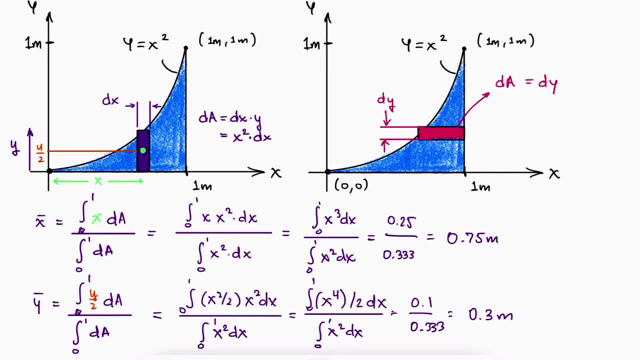 centroid would be at 0.3 meters and that the x-coordinate for the centroid y bar would be at 0.3 meters. For horizontal rectangles, for finding the centroid, the d-area element would be equal to dy times 1 minus x, which in terms of y would be 1 minus square root of y, The centroid term for each rectangle. 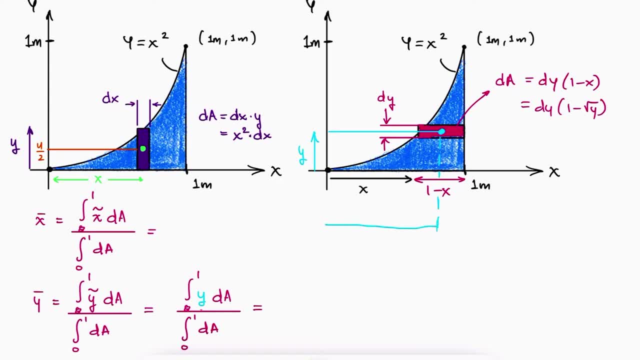 would be y for y bar and 1 minus half of 1 minus x for x bar, which results in 1 plus x over 2.. Substituting the variables, performing the integrals and evaluating from 0 to 1,. 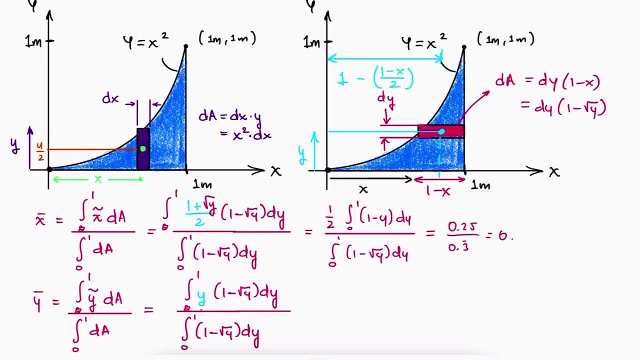 the boundaries of the area, we would still get a 0.5 meter square root of x. We would still get a 0.75 for x bar and a 0.3 for y bar. With this simple example, you can see that there is definitely a short and easy way. 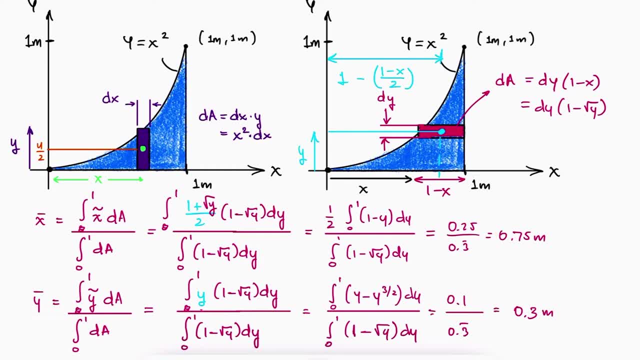 and a longer and harder way to find the same information. so always be wary of the math that you will have to carry out for either method: vertical or horizontal da rectangles. For your statics class, you'll most likely be asked to solve some problems like this. 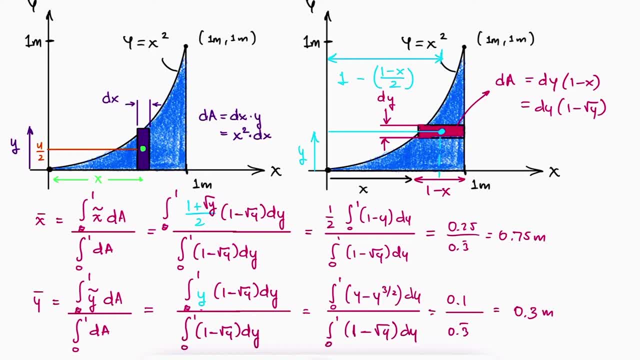 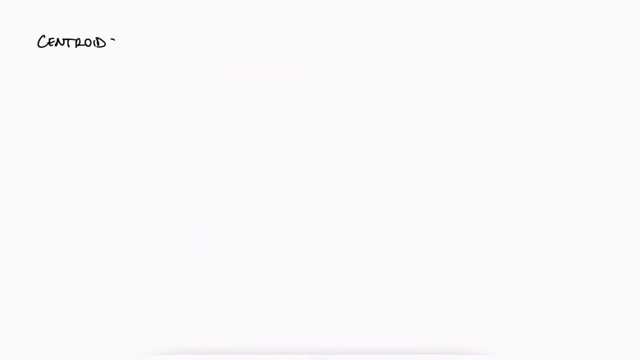 where a math function, fx, is given and you're asked to find the centroid For somewhat common geometries. the center of mass or the center of gravity will be somewhat helpful, but you'll find that what's most useful for structure-related calculations. 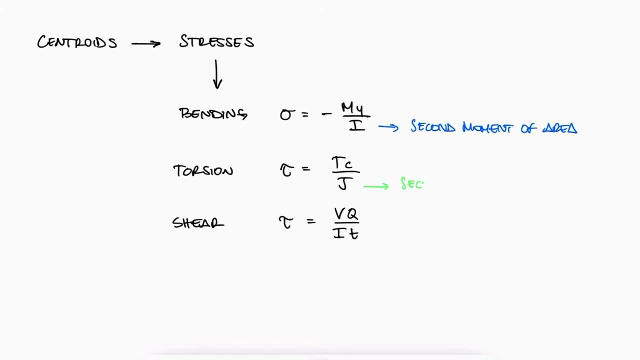 including stress calculations that require first and second moments of area in both Cartesian and polar coordinates, is the centroid of common shapes like rectangles, triangles and semicircles. Of course, you already know where the centroid for a rectangle is located, since it's pretty intuitive. We just found the centroid for a right triangle. 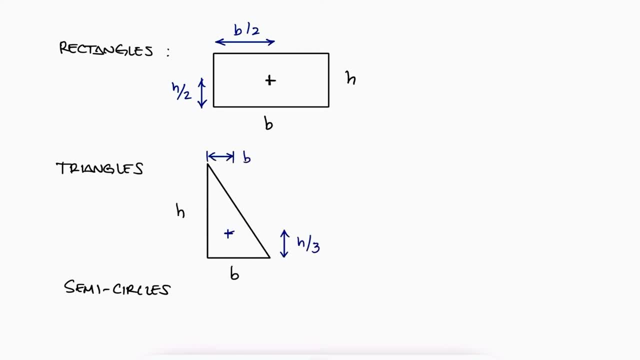 and if you perform the same process by changing the orientation of the triangle, it will still hold true. All we are missing now is the centroid of a semicircle, or what in practice is the same, a quarter of a circle. Using the circle equation, we see that for a quarter circle, 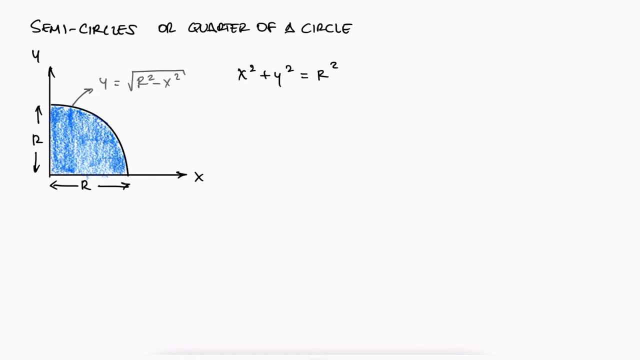 y is the square root of r squared minus x squared. The centroid of a rectangle at a distance x would be x and the d area term would be equal to dx times y. If we use our centroid equation to integrate x from 0 to r and substitute the variables with what we have, we find that x bar. 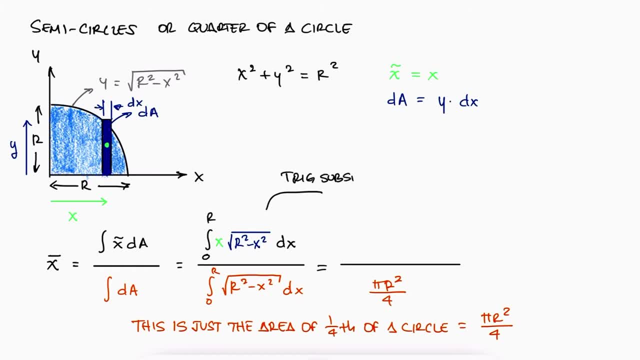 the centroid in the x axis from the center of the circle would be 4r over 3 pi. And since the x and the y axis are symmetric, this is true for y bar as well. Now, what about more complex shapes that? 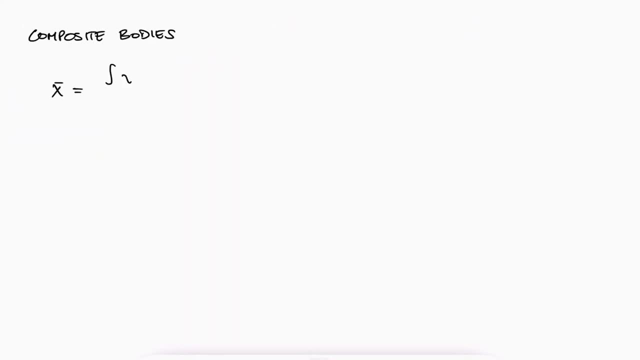 can be constructed from putting simple shapes together. All the main expressions we developed in terms of integrals can be used here, but instead of adding up an infinite number of differential weights, masses, volumes and areas, which is what the integral is effectively doing, we can instead have a finite number of weights, masses, volumes. 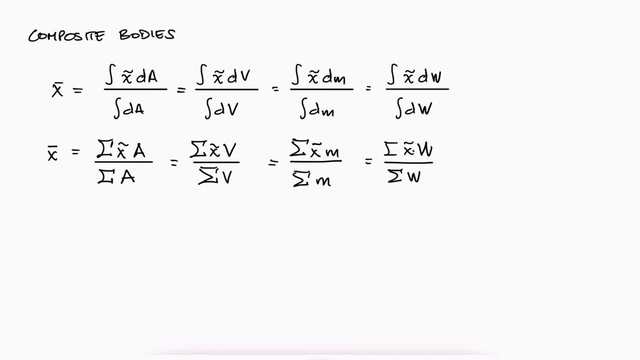 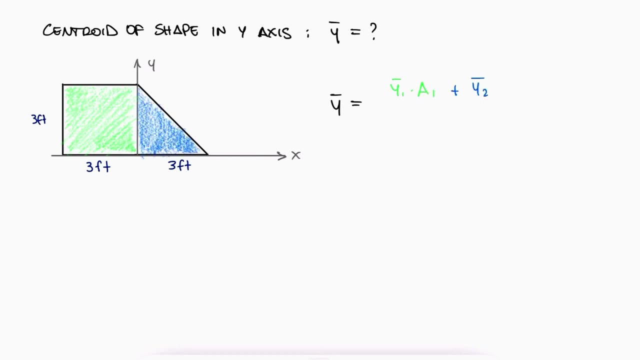 or areas, And that's why we write them as a sum instead of an integral. For example, if we are trying to find the overall centroid in the y axis, meaning y bar, of a shape that is formed by a square and a right triangle, y bar would be equal to y bar times. area of each shape. 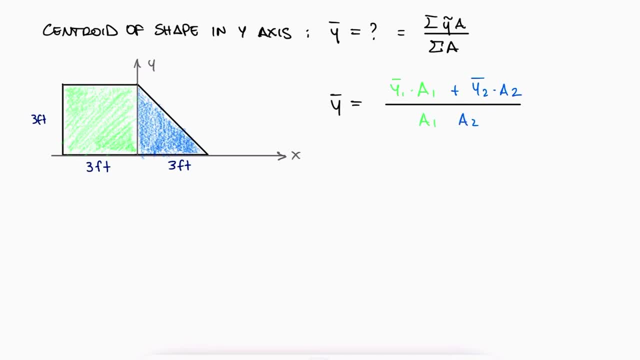 added together over the sum of the areas in the denominator. The centroid of the square is right in the middle, h over 2, and the centroid of the triangle is found at h over 3.. Of course, the datum or plane of reference. 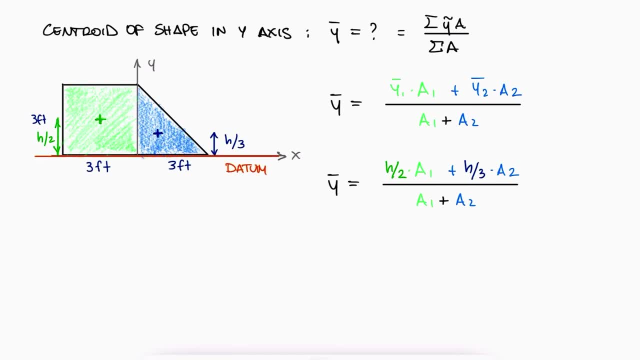 has to be the same for all shapes, And the values we obtain for y bar in this case, or x bar in the case where we are looking for the centroid along the x axis, will be the distances from that point of reference. Substituting the values, including the values for the areas, we find the overall 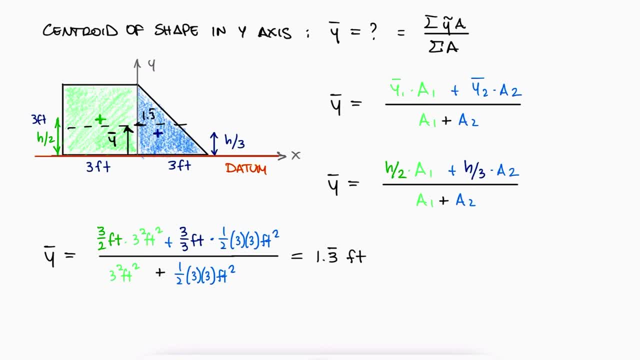 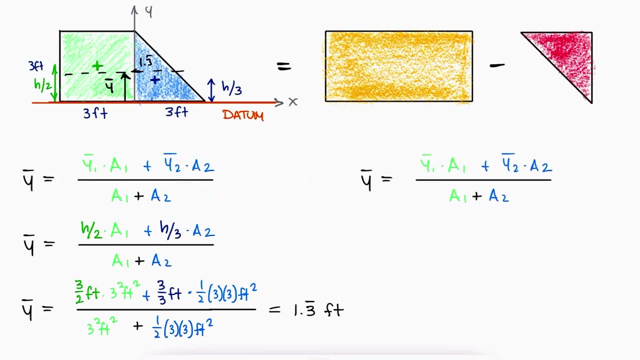 centroid of that more complex shape. Notice that the same shape can be obtained by subtracting a triangle from a larger rectangle. In this case, the sum expressions would of course include a negative sign for the triangle you're subtracting from the rectangle. The centroid of the rectangle. 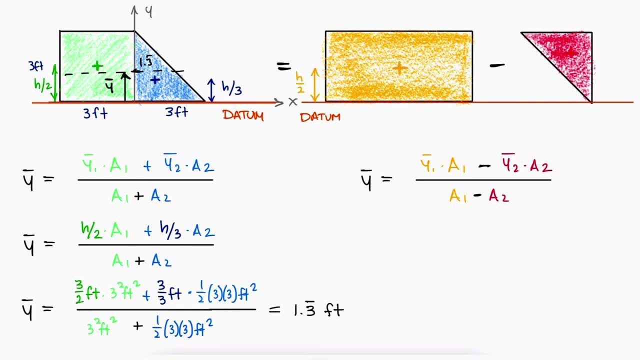 is still at h over 2, and the centroid of the triangle is at h over 3 from the top, meaning 2h over 3 from the bottom. our datum. And of course, always remember to have the same frame of reference for each of the two triangles. And that's it for this video, If you liked this video.